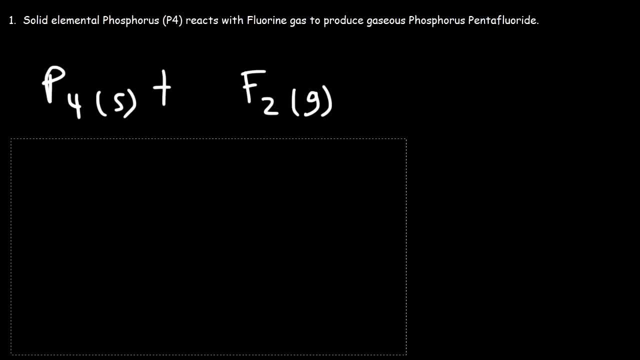 make sure you know those seven diatomic elements. Now, the product of this reaction is a hydrogen gas. Now, the product of this reaction is a hydrogen gas. Now, the product of this reaction is a reaction is phosphorus pentafluoride. Penta means five, So it's PF5.. And it's in a 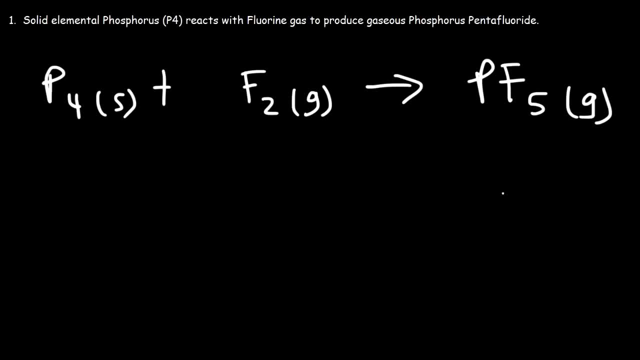 gaseous state. So that's the chemical equation that corresponds to the sentence. Now what we need to do is balance the chemical equation. So we have two elements that we need to concern ourselves with: Phosphorus and fluorine. So right now, on the left side, we have 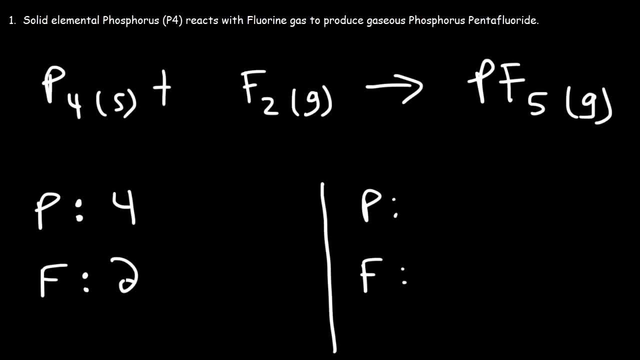 four phosphorus atoms and only two fluorine atoms. based on the subscript we see here On the right side, we have one phosphorus atom and five fluorine atoms. So let's begin by balancing the phosphorus atoms. So we have four on the 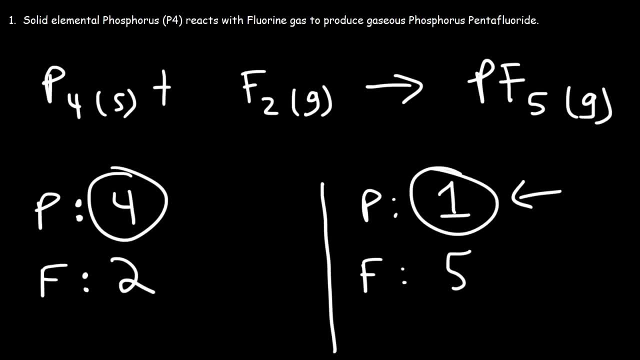 left, one on the right. So we need to multiply this number by four. So let's put a four in front of PF5.. So now we have four phosphorus atoms. Now the number of fluorine atoms they change. It's going to be four times five, which is 20.. So now we need to make this. 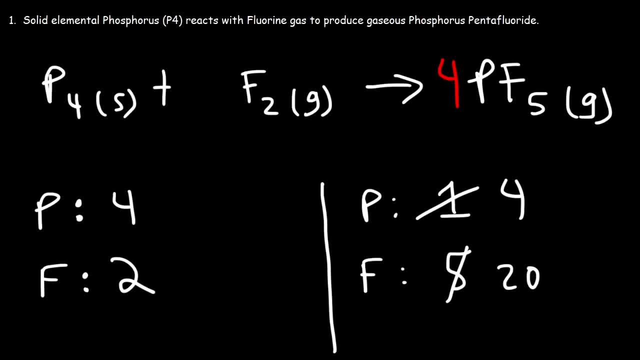 number 20.. Therefore, 20 divided by 2 is 10.. So let's put a 10 in front of F2.. So now this is going to be 20.. So we can see that the number of phosphorus atoms are equal, and also the number of. 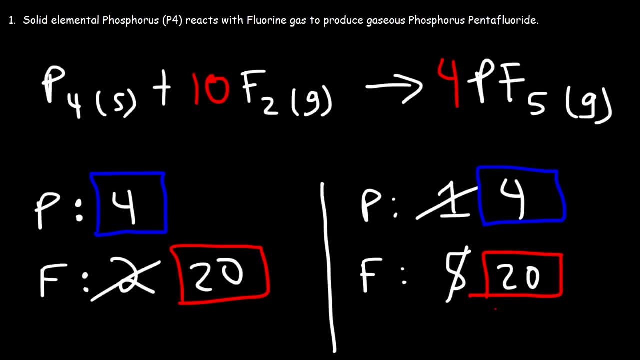 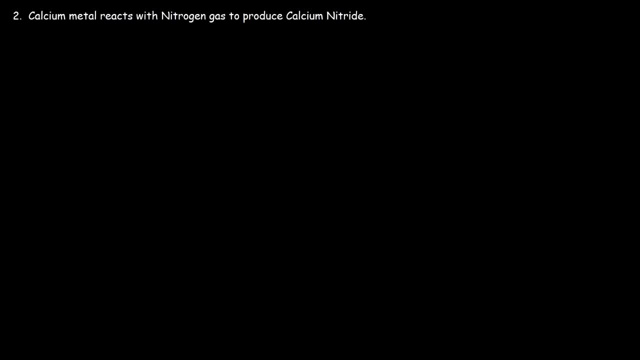 fluorine atoms are equal, And so that's it. So that's the balanced chemical equation that corresponds to this word description. Now let's work on this one. Number two: Calcium metal. so that's Ca, and metals are usually in the solid phase. calcium metal reacts with nitrogen. 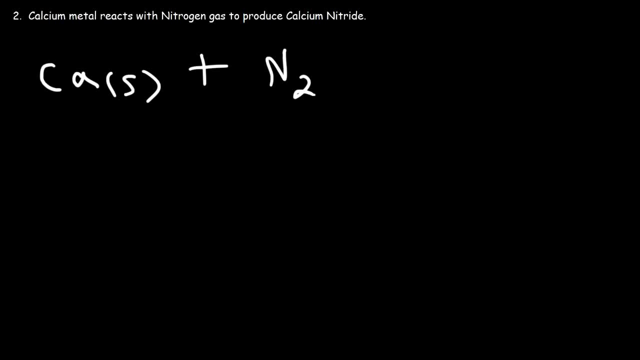 gas And, just as we mentioned before, nitrogen is a diatomic molecule to produce calcium nitride. Now, for these types of problems, you need to be able to write the formula of a chemical compound. So this is an ionic compound and therefore we need to write. 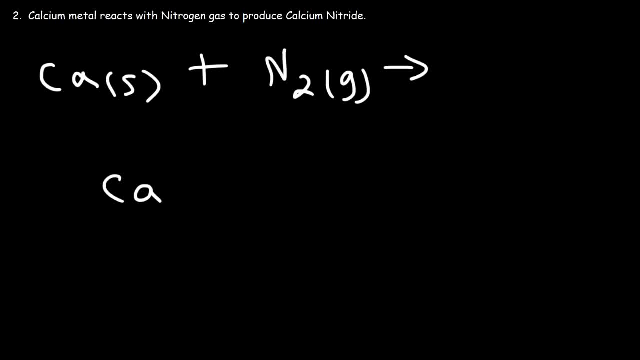 the ions. first, Calcium exists in group IIa, so it has two valence electrons As an ion. it's gonna have a two plus charge Nitride- existing group 5a or group 15a- and so it needs it needs three more electrons to 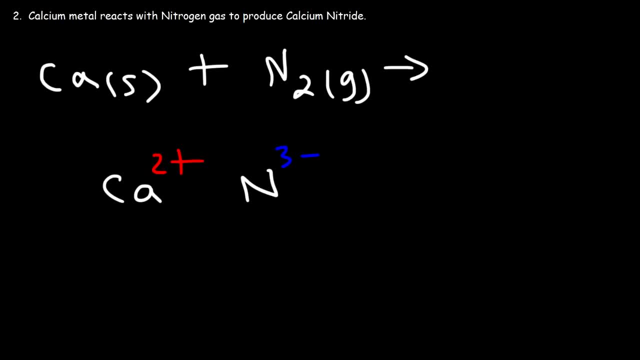 get to eight, so those ions typically form a negative 3 or 3 minus charge. now perhaps you've seen this method where you can replace the charges with subscripts, and if you use it you'll get this formula: CA3 and 2, and so that is. the formula for calcium nitride. for those of you who wish to understand why this works, what we need is three calcium ions and two nitride ions. the reason for this is charge balance. the sum of the positive charges must equal the sum of the negative charges, and so if you add two, three times, you're going to get six. 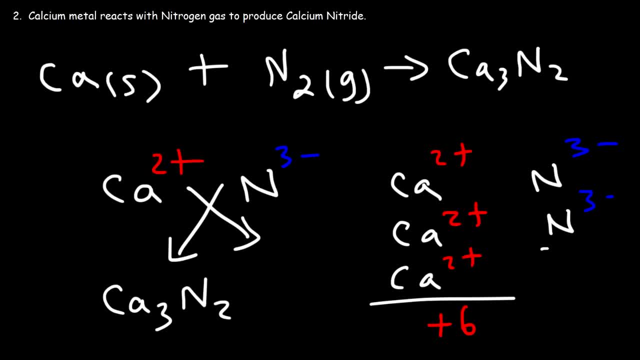 or if you add 32 times, you also get six. in this case, two negative threes will add up to negative six, and so that's why we need three calcium ions and two nitride ions to balance out all of the positive and the negative charges. but if you use 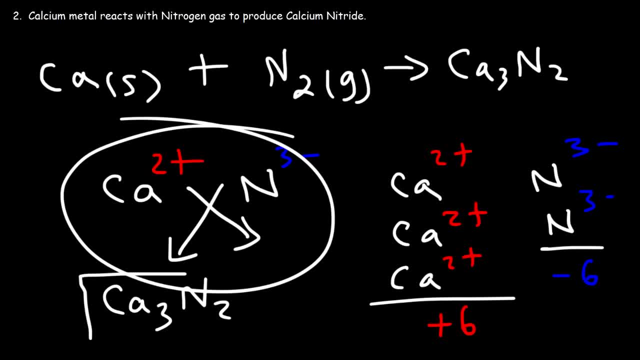 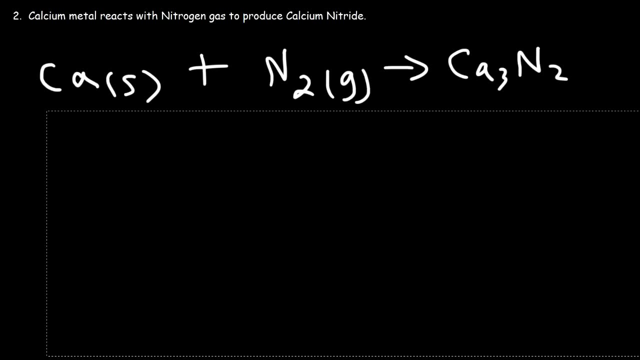 this crisscross technique you can quickly get the answer. so this three becomes the subscript here and this charge of two becomes the subscript of the negative charge. as you see on the right side now is calcium nitride a solid liquid or a gas. how are we supposed to know if it's not given to us in the sentence? now, you know. 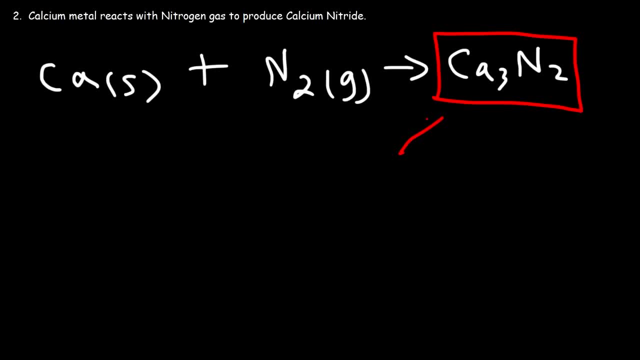 this to be an ionic compound, which is between a metal and a nonmetal, and that's usually the case. there are some exceptions, but a compound consistent of ions is an ionic compound, and most ionic compounds, almost all of them, but a high percentage of them exists in a solid form. so 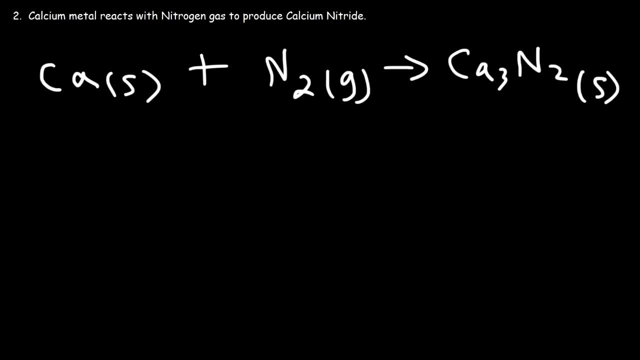 therefore, calcium nitride is going to be a solid, if anything. you can look it up on the internet to see if it's a liquid solid or something like that. now let's go ahead and balance the equation. if you want to pause the video, feel free to do. 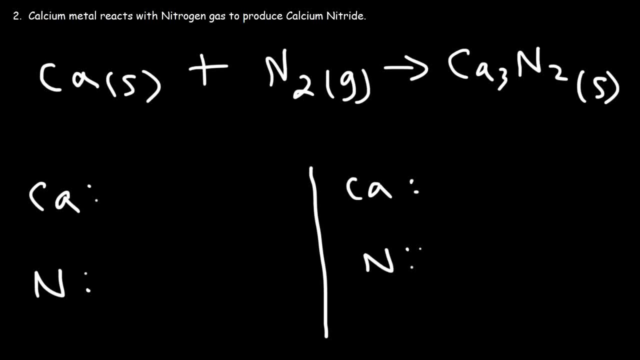 so if you want to try this yourself. so on the left side we have one calcium atom and two nitrogen atoms. on the right side we have three calcium atoms and two nitrogen atoms. so the nitrogen atoms are already balanced, so we're not going to worry about that. now we need to multiply the number of calcium atoms by three, so 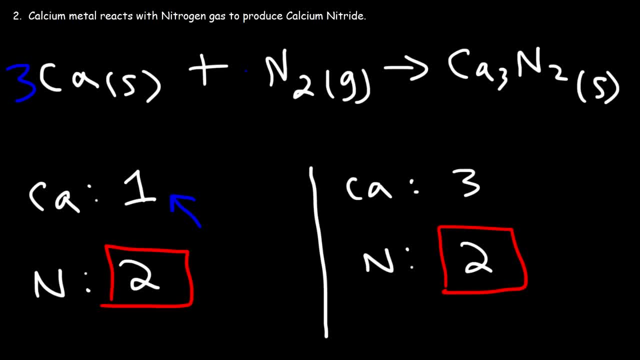 let's put a three in front of CA. if you want to, you can put a coefficient of one. you really don't need it there, but you could if you want to. and so now we're not going to have one calcium atom on the left side, but three, and so the number of calcium atoms are. 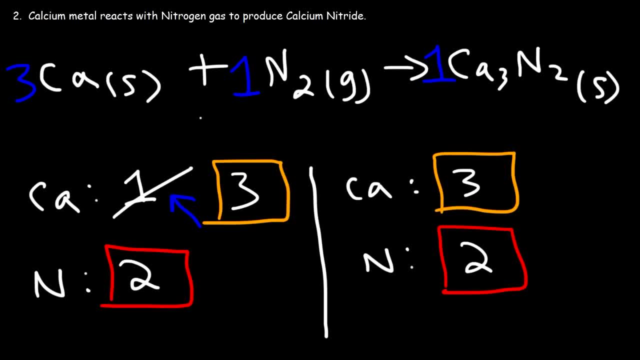 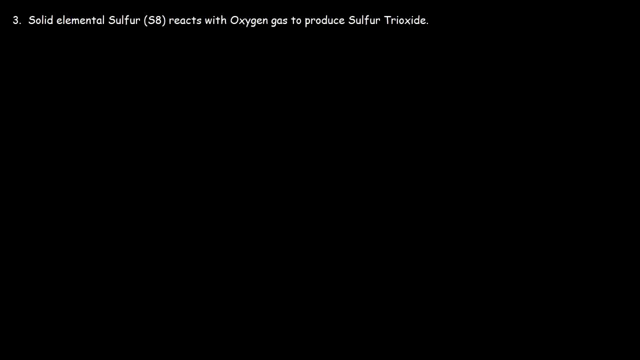 equal as well, and so this right here is the balance chemical equation for this word description. here's another one that we could try: solid elemental sulfur, so that's s8, and the phase is solid, as the sentence depicted. it reacts with oxygen gas, so we know that to be o2, to produce sulfur trioxide, now sulfur. 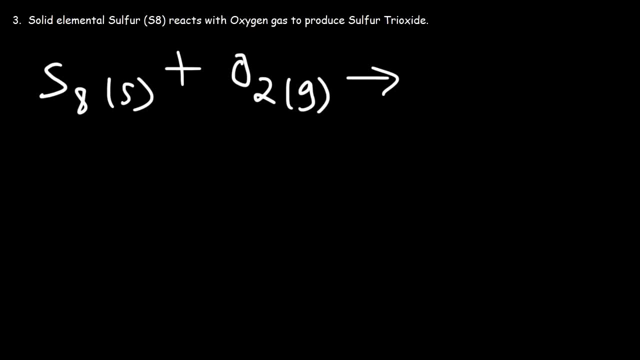 trioxide is a compound because it's made up of different elements and this is not an ionic compound. if you see the words di tri, tetra or Penta, things like that, you know you're dealing with a covalent molecular compound and the fact that it 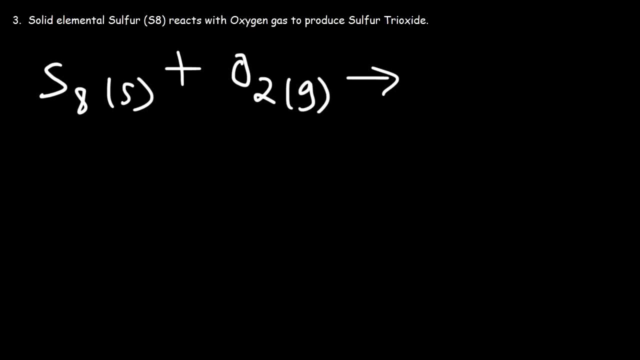 consists of non-metals. sulfur and oxygen are non-metals. but this you don't need to use that crisscross method that we did in the last example. you can simply write S for sulfur and O3 for trioxide. tri means three. now sulfur trioxide is a. 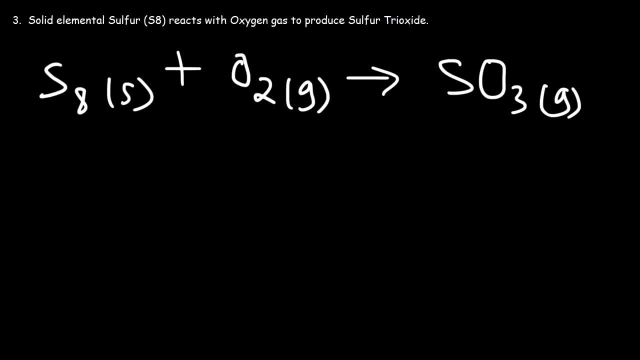 gas. I forgot to write gaseous sulfur trioxide, but you can look that up: sulfur dioxide, in case you see it. that's also a gas. now let's go ahead and balance the chemical equation. so on the left we have two- I mean eight- sulfur atoms, but two. 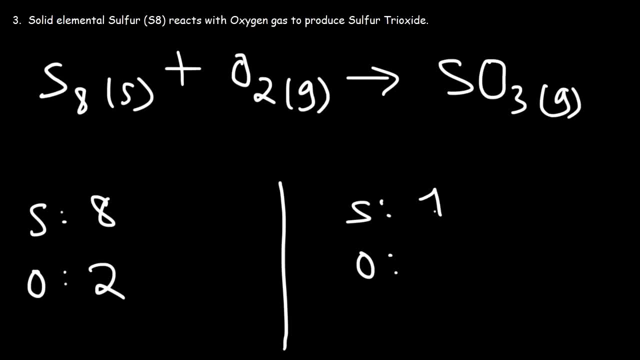 oxygen atoms. on the right we have one sulfur atom- there is an invisible one as a subscript here- and three oxygen atoms. so let's begin by balancing the sulfur atoms first. So we need to put an 8 in front of SO3.. So now we have 8 sulfur. 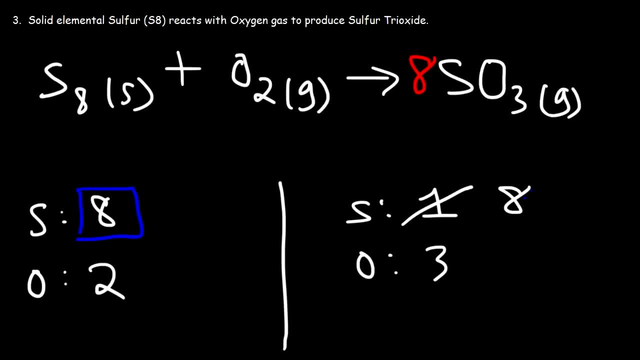 atoms on the right side. So these two are equal and the number of oxygen atoms will change. now It's going to be 8 times 3, which is 24.. So we have 24 oxygen atoms on the right side. Now, 24 divided by 2 is 12.. So let's put a 12 in front of O2.. And if you want to, 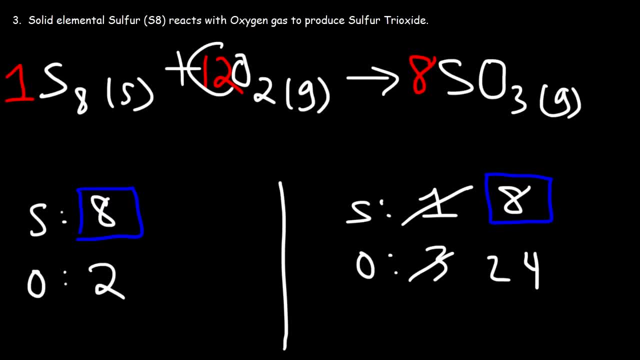 you can put a 1 in front of S8. So here, 12 times 2 is 24.. And so the number of oxygen atoms are the same. now, And that's it. That's all we got to do for this example, And so. 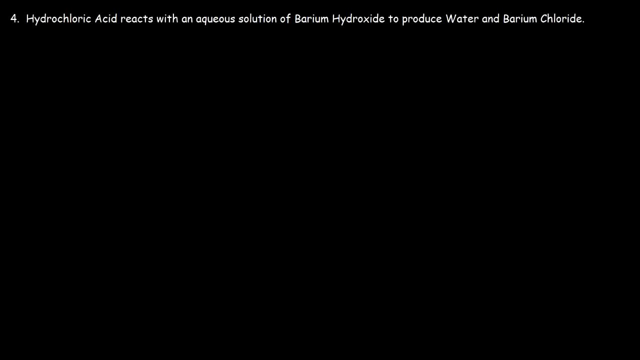 now we have our balance chemical equation. Now for this type of problem, we're going to need to put an 8 in front of O2.. So we need to be familiar with the solubility rules, And I'm going to post a link in the description. 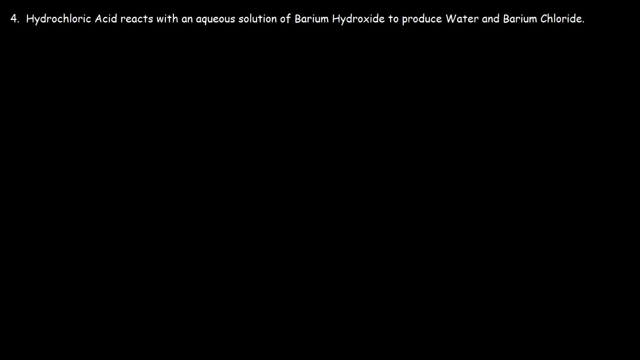 section of this video to another video where you can learn the solubility rules if you need to: Hydrochloric acid. So what is that? What is the chemical formula for hydrochloric acid? You need to know that it's HCl. I would commit that one to memory, And most 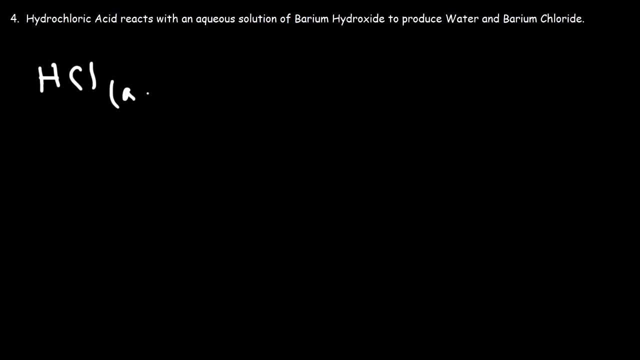 of the time, you're going to need to know that it's HCl. So you need to know that it's HCl In principle. you need to know that. it's very important to know that it's HCl. And, as we're gathering all these acids, I don't know if any of that are not, But acids. 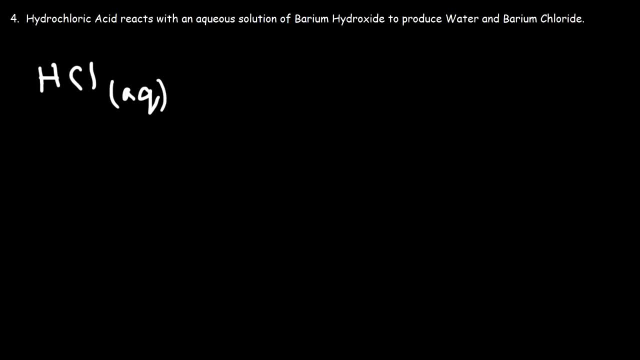 are usually soluble in water, So we're going to put it in the aqueous phase. Next we have barium hydroxide and we're told that it's aqueous, so it dissolves in water, And you could find that out from the solubility rules. Hydroxides are usually soluble in group 1. 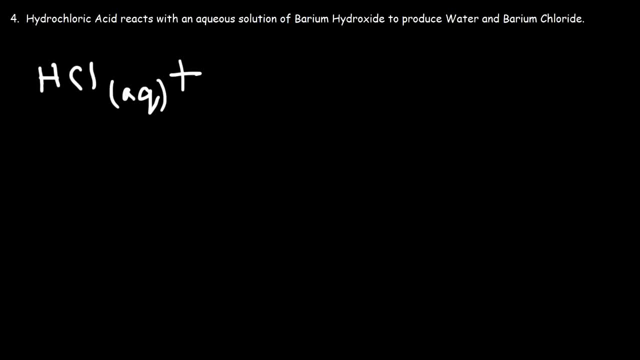 and for the heavy elements in group 2.. But because this is an ionic compound, barium is a metal. Hydroxide is an atom, So it dissolves in water. For any of you that's familiar with a nonmetal, We need to write the formula for it using that crisscross method. Barium has a 2 plus. 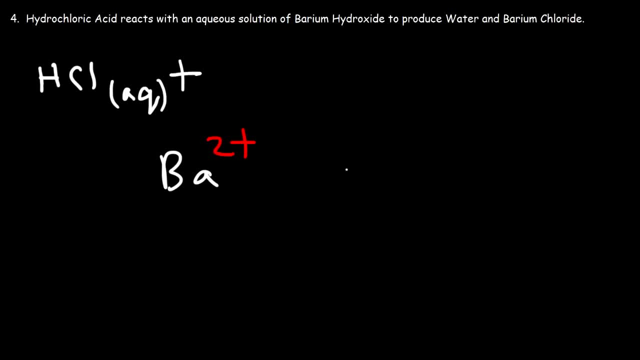 charge. Hydroxide is a polyatomic ion and so you also need to memorize the polyatomic ions, which I'm going to post a link in the description section to help you out with that. Hydroxide has a minus 1 charge, So using the crisscross method, it's going to be Ba1OH2.. Whenever you 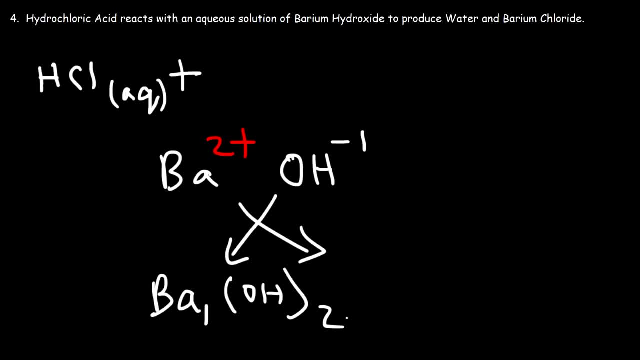 have multiple polyatomic ions, you need to enclose it within a set of parentheses. So this is BaOH2 and it's in the aqueous phase. Now let's move on to the product side of this reaction. So we have water. 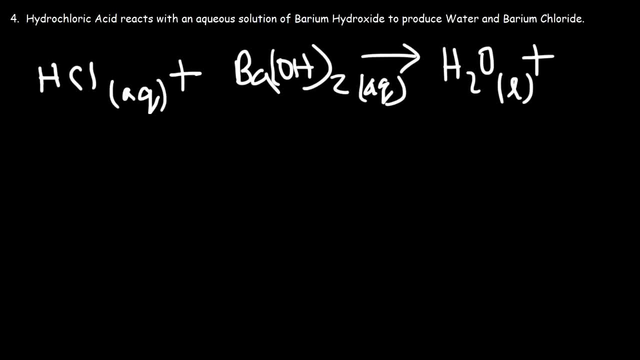 We're going to assume that it's in a liquid state Plus barium chloride, So we need to use the crisscross method. Chloride is a halogen which all have a negative 1 charges as an ion. So, using the same method, it's Ba1Cl2.. We're simply BaCl2.. 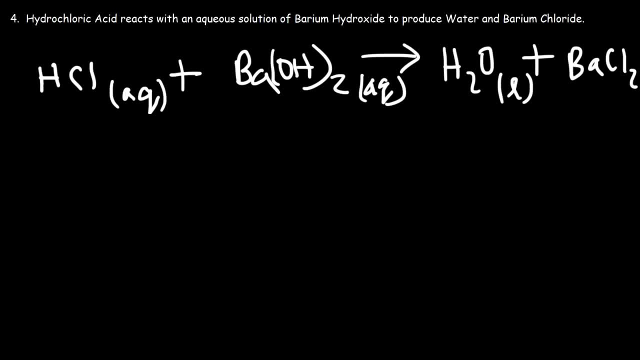 Now BaCl2, Barium chloride, BaCl2, is it soluble or is it insoluble? Does it dissolve in water or will it not? So should we write aqueous or solid? So here's when you need to know the solubility rules. 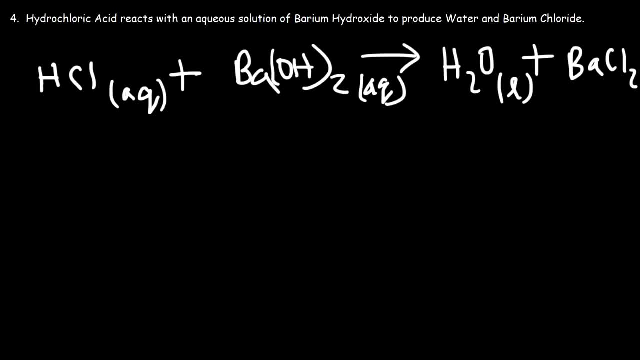 Chlorides are generally soluble, except with silver, lead and mercury. Since it doesn't have one of them, therefore, BaCl2 is soluble, which means that it dissolves in water. so we're going to write aqueous. It will exist in the aqueous phase. 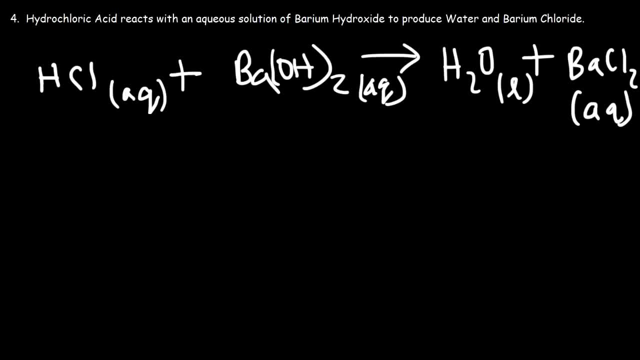 And so that's it for this particular chemical reaction. Now, sometimes you may be given a word description without the products of the reaction. In this video I've given you the entire chemical reaction, The reactants and the products, But sometimes you need to predict the products yourself. 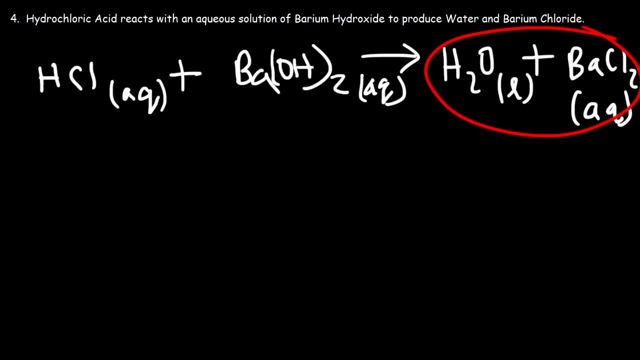 And this type of reaction is a double replacement reaction, And so not only do you need to know what type of reaction you're dealing with, but you also need to know how to predict the products of the reaction, And the methods by which you would do so varies on the type of reaction you're dealing with. 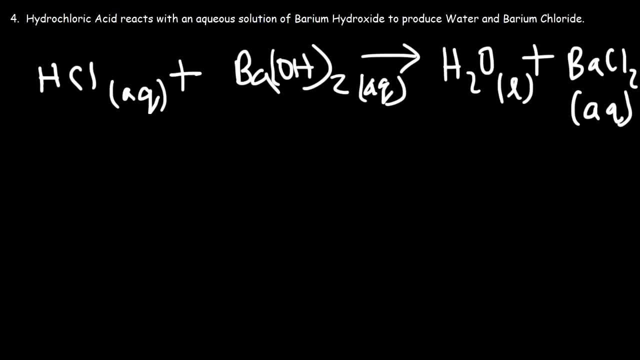 So I'm going to post some other links to this video: One, how to predict the products of chemical reactions, And two, how to distinguish between the different types of chemical reactions that are out there. So it might be useful for you to watch both of those videos when you get a chance. 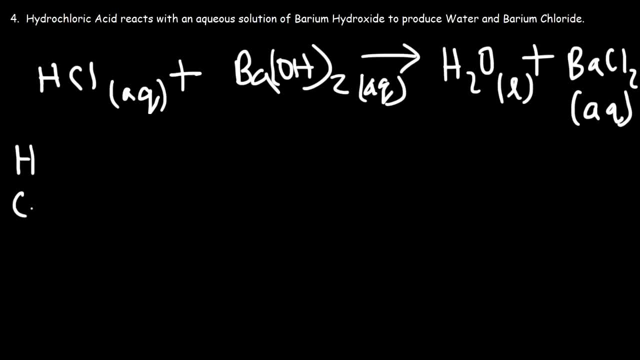 Now let's work on balancing the chemical reaction. So let's write the elements that we have. We have hydrogen, chlorine, barium and oxygen, So let's write it again. on the other side of the reaction, So let's write the elements that we have. 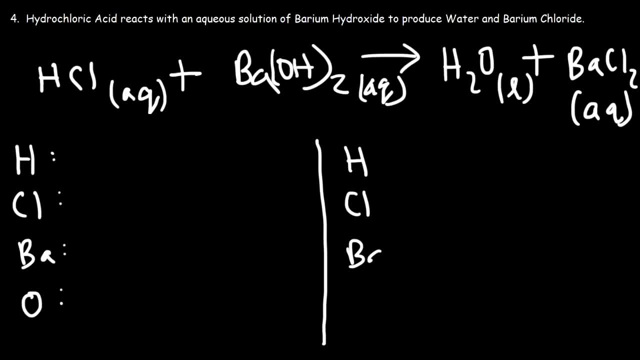 We have hydrogen, chlorine, barium and oxygen. So let's write it again on the other side of the reaction. So let's write it again on the other side of the reaction. On the left side right now we have a total of 3 hydrogen atoms. 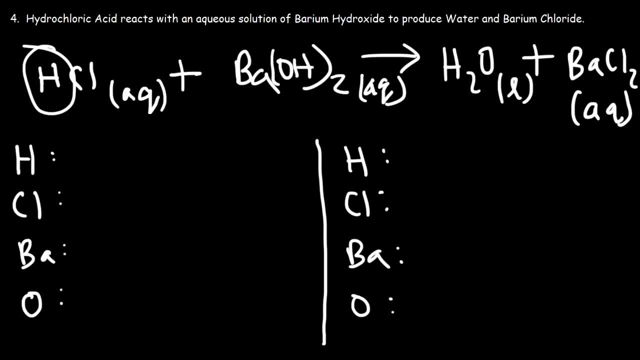 We have 1 in HCl but 2 in barium hydroxide, So we have 3.. And we have 1 chlorine atom in HCl, 1 barium atom in BaOH2, and 2 oxygen atoms, So we have 3.. 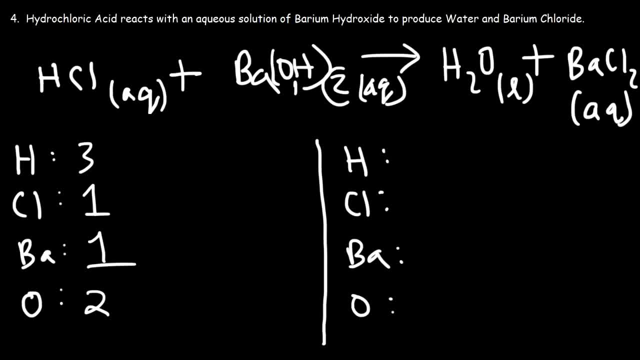 And we have 1 chlorine atom in HCl, 1 barium atom in BaOH2, and 2 oxygen atoms, 1 x 2.. On the right side we have two hydrogen atoms in water, two chlorine atoms in BACL2, one. 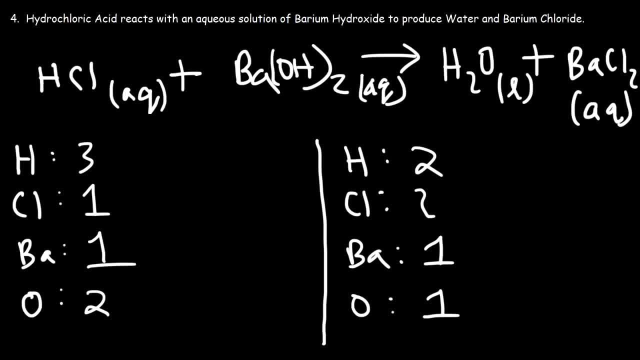 barium atom and one oxygen atom. So the first thing I'm going to do is: well, right now, notice that barium is already balanced, so we don't have to worry about that. but let's balance the chlorine atoms now. 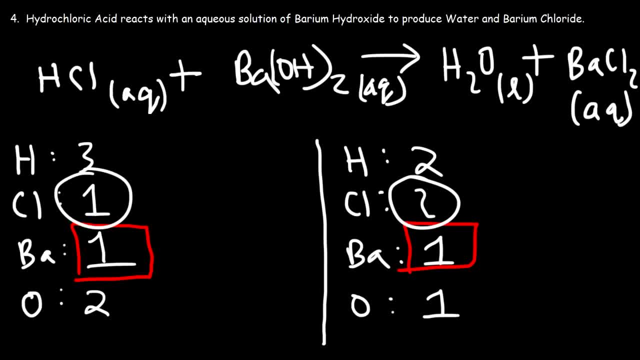 Notice that we have two chlorine atoms on the right side, only one on the left. So let's put a 2 in front of HCl, So this becomes 2, and so these two are now equal. However, the number of hydrogen atoms changes. 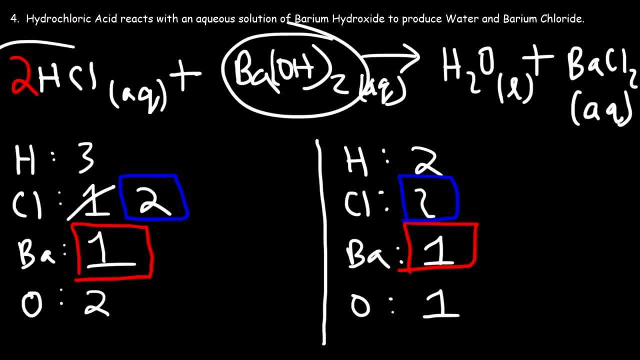 We have two hydrogen atoms in BaOH2, and two in HCl. 2 plus 2 is 4.. So now we need to make this work. We need this number of 4.. The only way to do that is to put a 2 in front of H2O. 2 times 2 is 4.. 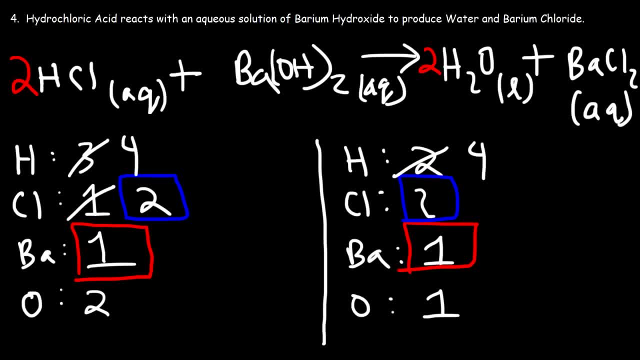 So now we have four hydrogen atoms And now the number of oxygen atoms will change. on the right side This is 2 times the invisible one, and so we have two oxygen atoms. So these two are equal and the number of hydrogen atoms are equal. 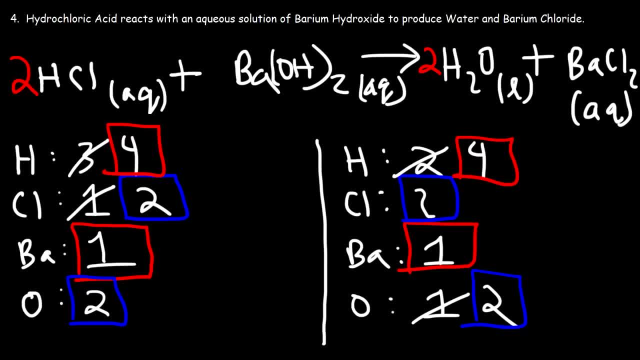 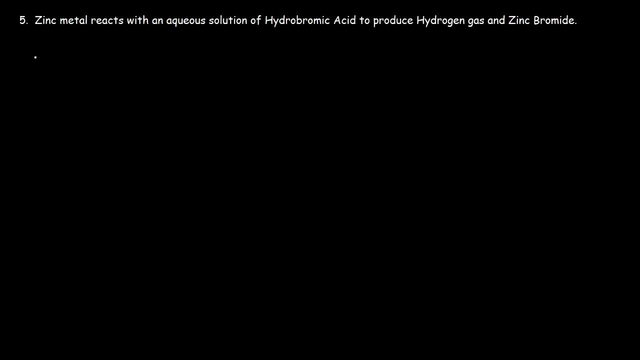 So now the equation is balanced. Now here is another one that you could try. Feel free to pause the video and work on it. So we have zinc metal, So it's in a solid phase. It reacts with hydrobromic acid. 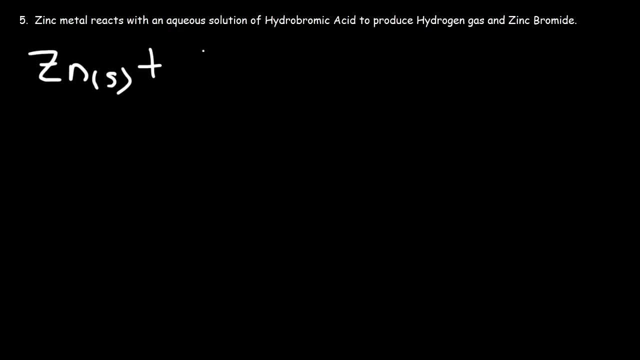 Now recall that hydrochloric acid is HCl. Therefore hydrobromic acid is HBr And it's in the aqueous phase And it's going to produce hydrochloric acid And it's going to produce HCl- Hydrogen gas, which is diatomic, and zinc bromide. 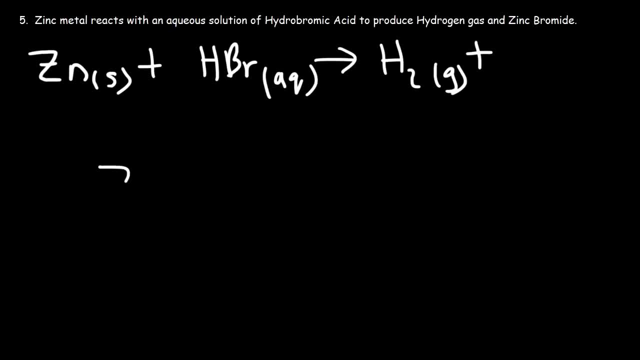 Now this is an ionic compound, so let's write the chemical formula. Now you need to know that zinc has a 2 plus charge 99% of the time. Bromide has a minus 1 charge. So, using the criss-cross method, it's going to be Zn1Br2, but we don't need to write the 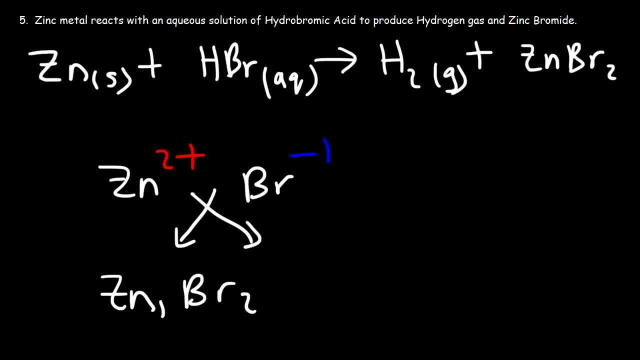 1.. So ZnBr2.. And halides are generally soluble except with silver, lead and mercury. So zinc bromide dissolves in water. It's soluble, which means that we're going to write it in the aqueous phase. 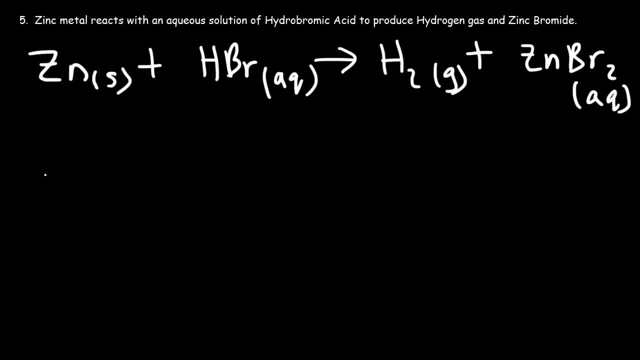 Now let's go ahead and balance the chemical reaction. So we have zinc hydrogen and bromine. By the way, do you know what type of reaction this is? What type of reaction are we doing? What are we dealing with here? 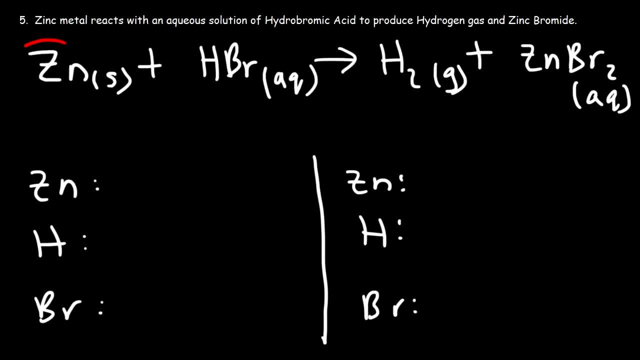 This is a single replacement reaction. Zinc replaces hydrogen in this particular reaction. It displaces hydrogen, So zinc pairs up with bromine, causing hydrogen to be by itself. So thus this is a single replacement reaction. Now, when predicting the products of a single replacement reaction, you need to be familiar. 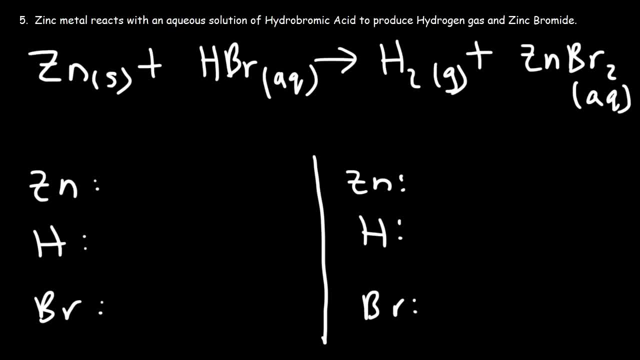 with the activity series. Zinc is more active than hydrogen, and that's why it could displace it, And so this chemical reaction would occur. Copper is less active than hydrogen. If copper were here instead, there would be no reaction, And so if you're given a question like this without the products, you need to reference. 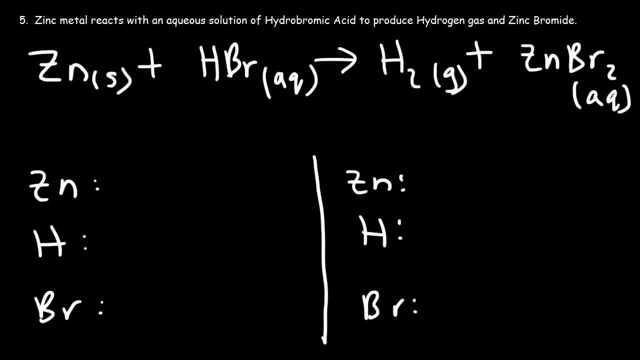 the activity series which I'm going to post in this video as well. So right now we have one zinc atom on the left side, One hydrogen atom and one bromine atom. On the right side we have one zinc atom, two hydrogen atoms and two bromine atoms. 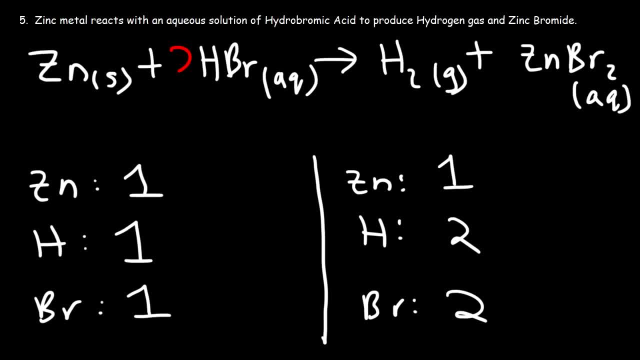 So let's begin by balancing the bromine atoms. Let's put a two in front of HBr, So this will change to two, and so will that one. So, automatically, the number of bromine atoms are the same, And also the number of hydrogen atoms are the same. 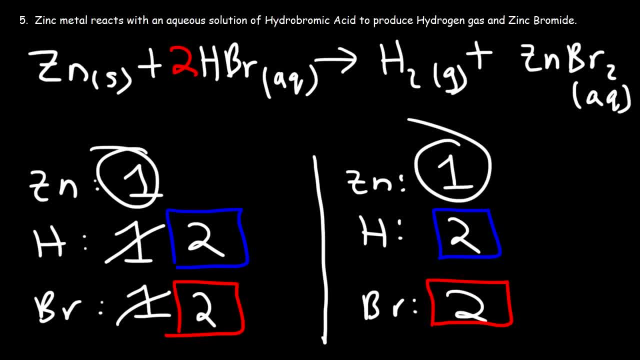 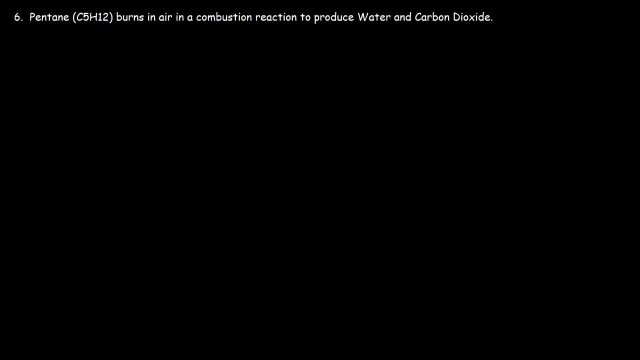 And already the number of zinc atoms are the same, So this is a single replacement reaction. atoms are the same, so that's all we got to do. The chemical reaction is balance. Now let's move on to number six. the last one: Pentane, C5H12,, and pentane is a liquid. 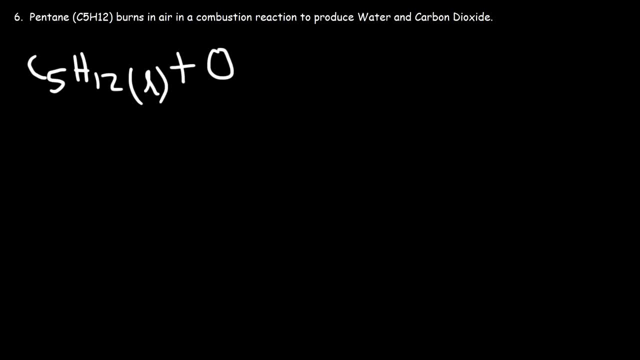 so let's put L. It burns in air, which means that it reacts with oxygen gas in the air to produce water. Now, granted, at high temperatures a liquid water becomes steam, but let's say it's just liquid for now. And carbon dioxide, CO2, that's a gas. 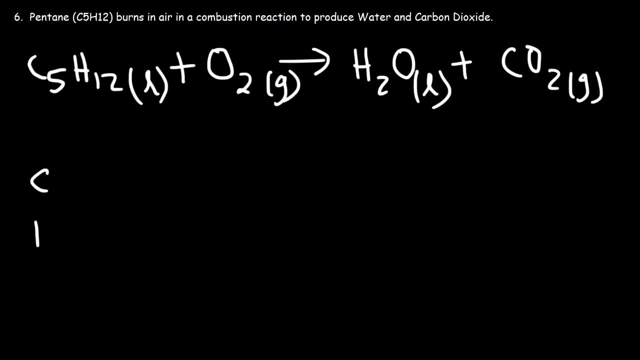 So now let's go ahead and balance the chemical reaction, So this is called a combustion reaction. Now for this. it's expected that you know the products of a combustion. This is a combustion reaction, which is always carbon dioxide and water. When balancing a combustion reaction, it helps to balance the carbon atoms first.